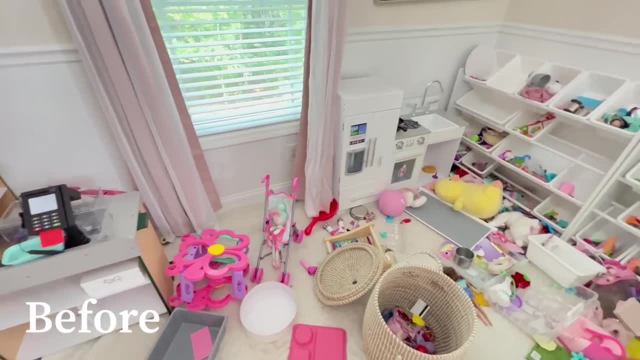 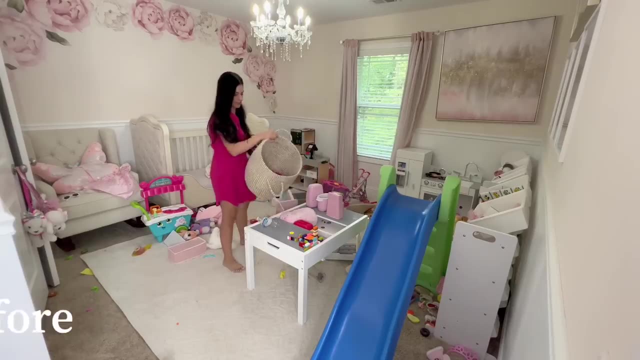 Today's another edition of my room makeover videos, where I'll be turning one of the existing rooms into a playroom. Now I know you may be thinking right now: why did I let my kids make this room a complete disaster? But I'm here to tell you guys the complete truth, Being a mom of three kids who are all under five years old. 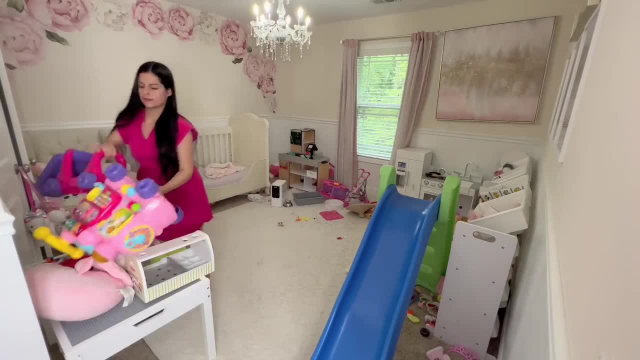 keeping room tidy in me is nearly impossible all of the time. This is what happens every now and then in a real view of behind the scenes. Now, don't let this scare you if you're soon to be a parent or want children someday. 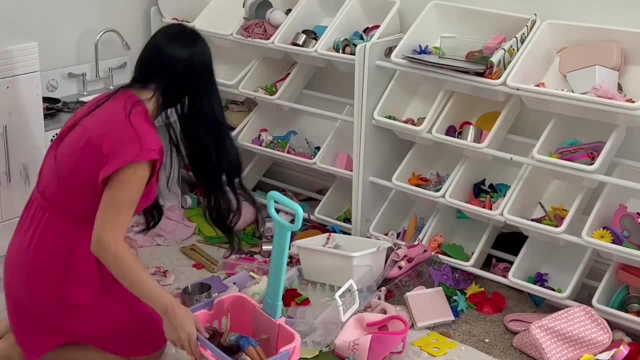 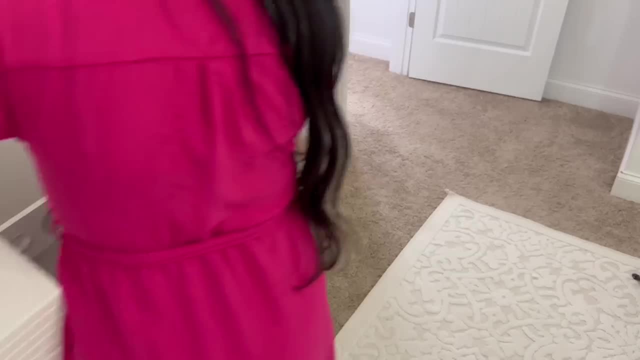 Trust me, they're all worth it and a tremendous blessing. I'm here today hopefully to give you some inspiration and motivation to tackle your very next project, and I'm also going to give this space a complete overhaul. Please stay through it all to see how we transformed and to see all of the details. 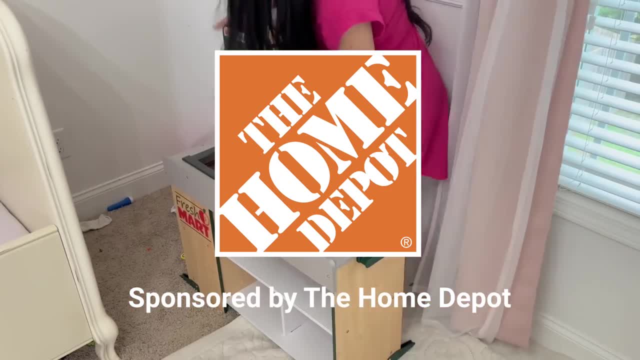 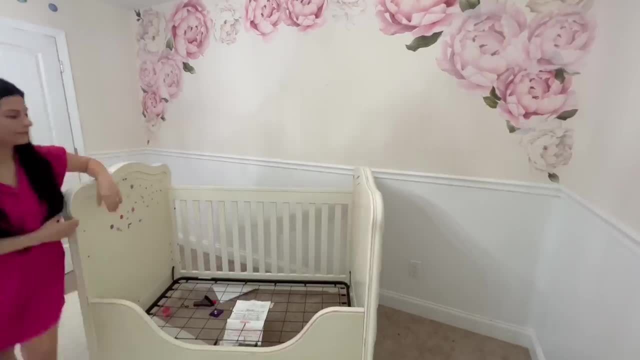 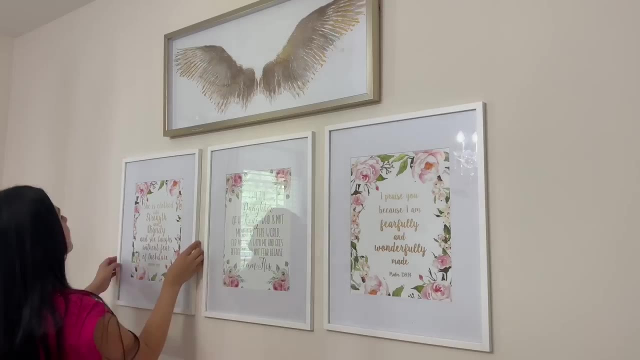 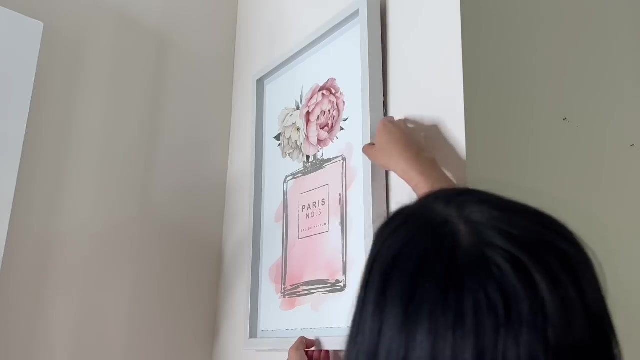 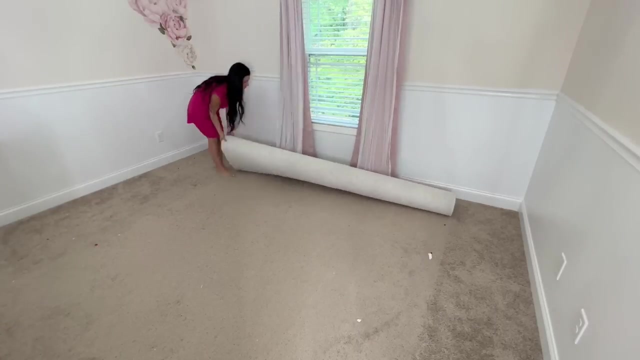 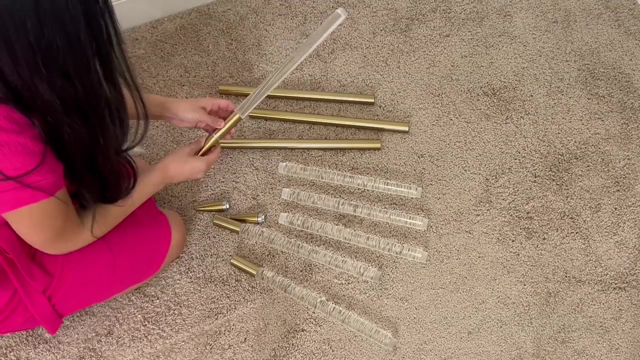 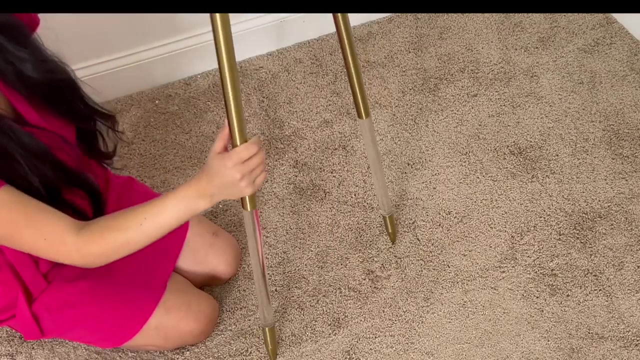 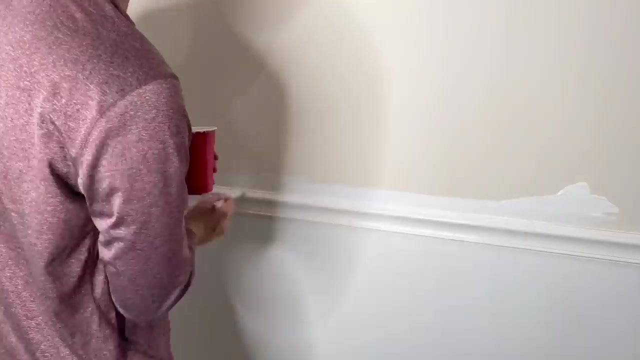 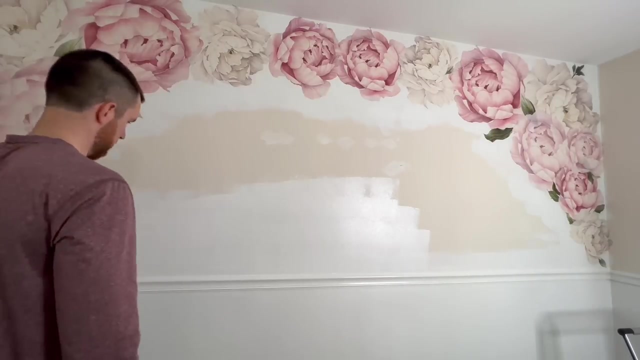 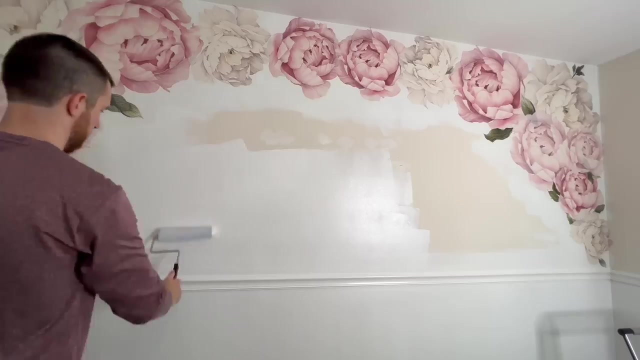 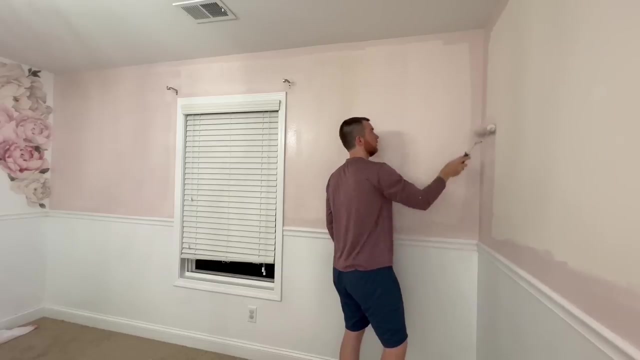 A huge thank you to The Home Depot for sponsoring this video. Thank you so much for watching and I'll see you guys in the next video. Bye To have completed the vision for my girls' playroom makeover. I couldn't have done it without the incredible unnecessary necessities. 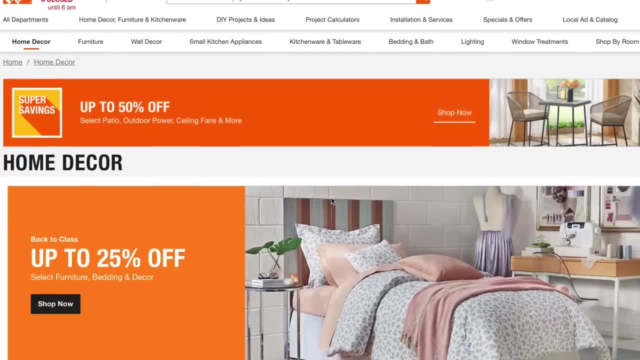 that I found shopping online from The Home Depot. I'm sure many people out there watching would think that The Home Depot is just a tool and hardware store, but that's not true at all. you guys, I've got some awesome things to share with you all. 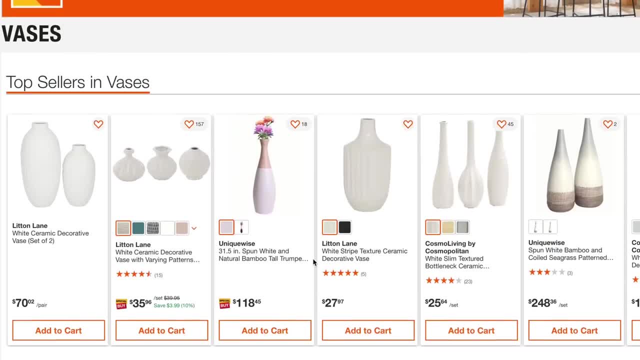 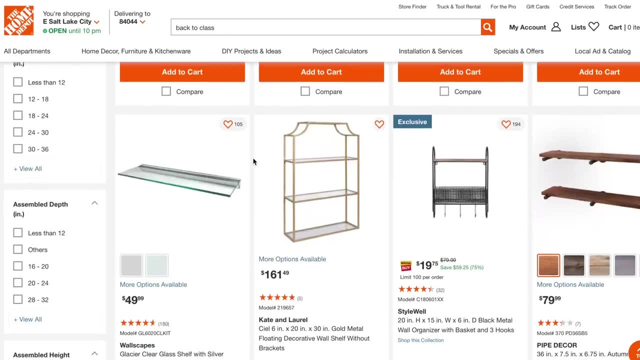 They literally have endless options Decor that's only online, and I'm so amazed of what I've been able to find. The timing of this makeover is also so perfect because it's such a special time in our lives. I know many of you watching can remember when I announced my first pregnancy with my daughter years ago. 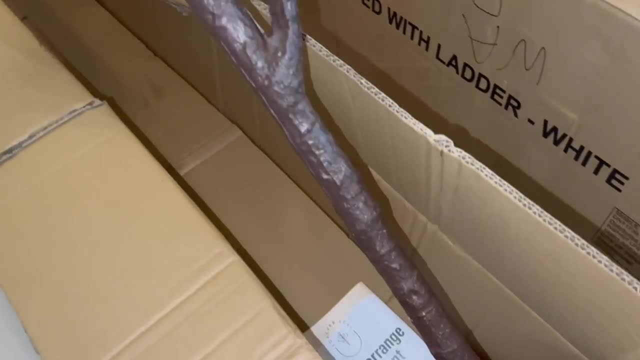 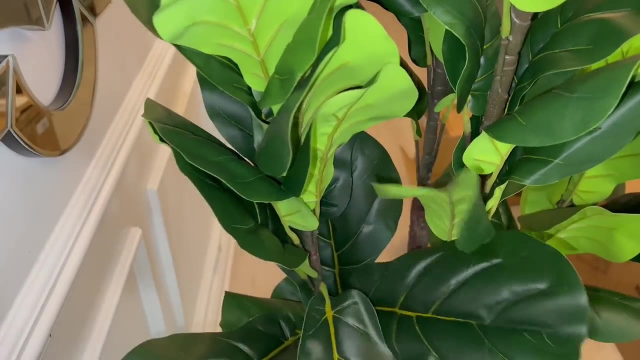 Can you believe we just enrolled her into kindergarten, With her going to learn and me giving her and her sister space of makeover. The Home Depot actually has a back-to-class promotion going on right now. that includes furniture, bedding and decor. I knew I wanted a fiddle leaf tree in a corner of their playroom to create an organic and cozy environment. 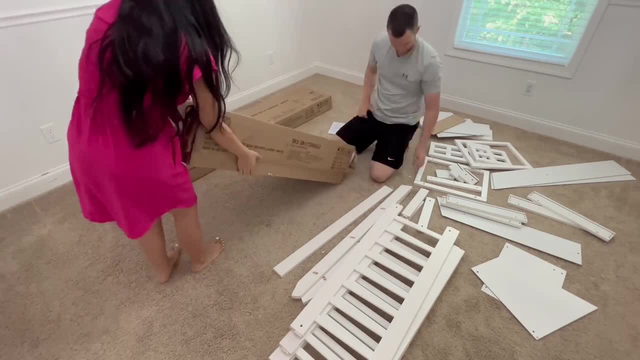 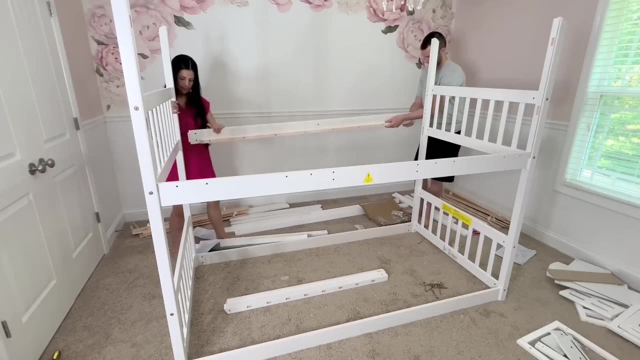 This one was so beautiful That I had to have it. when I first saw it online, I quickly took advantage of this promotion that's running and ordered several items from their website. You'll see how they really made this space come to life. I couldn't click fast enough to add this adorable bunk bed into the cart. you guys. 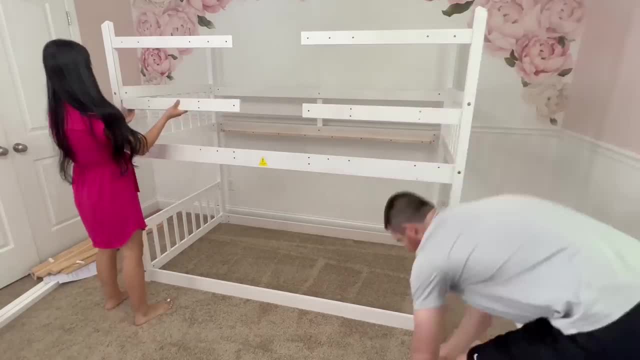 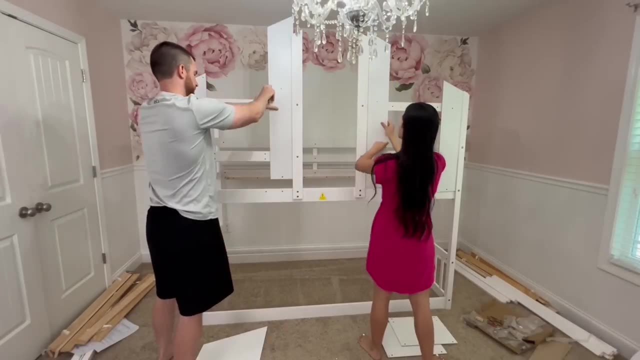 We went on vacation to the mountains last year and we stayed at a resort that had a bunk bed. Our girls got so much joy and excitement sleeping on it It was on our list to eventually get one for them. You all wouldn't believe how many times my girls asked when the room was going to be finished so they could sleep in it, play, study and have tons of fun. 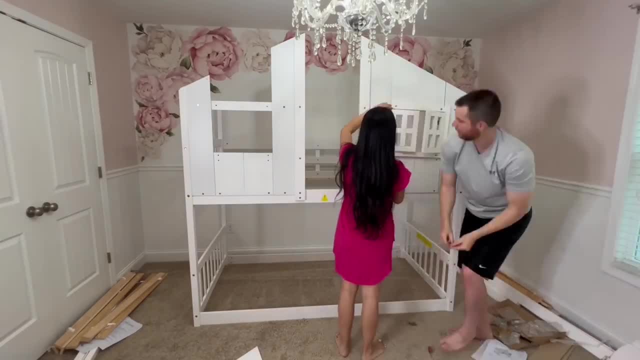 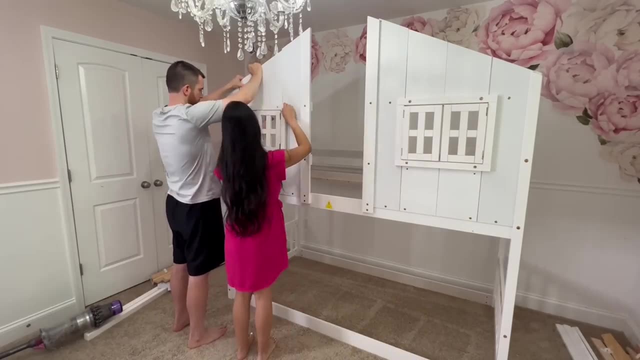 I know my girls will be sleeping there eight hours like princesses, And this bed to even out the backpack carrying they will be doing every day. The Home Depot is a trusted brand for home improvement And customers get the same experience when they shop furniture and decor for their DIY projects or home furnishings. 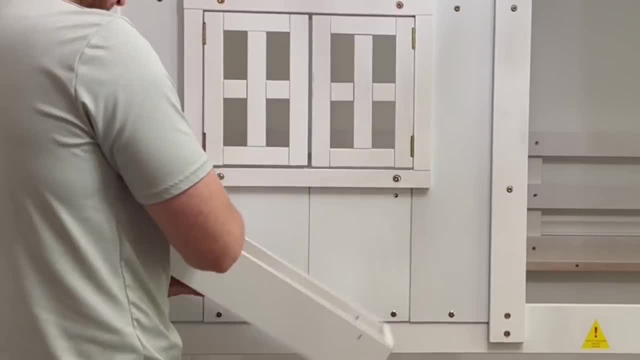 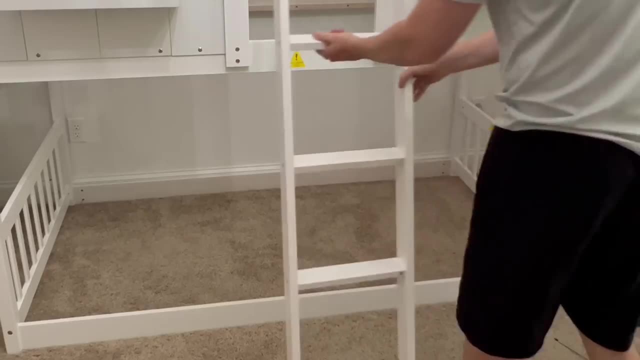 This was exactly the experience for me. I absolutely love everything I shopped online for and admire the quality and know they will last for years to come. Shopping online gets even better because it saved me time and there's also free delivery and flexible return options. 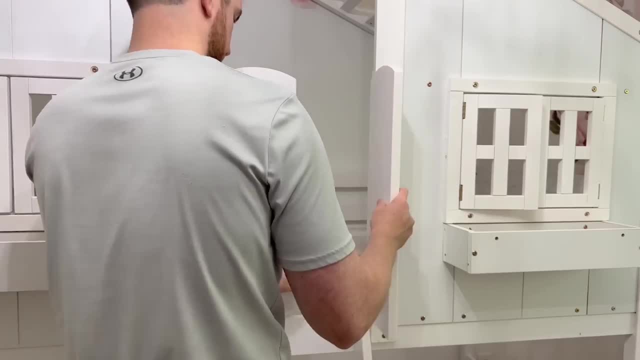 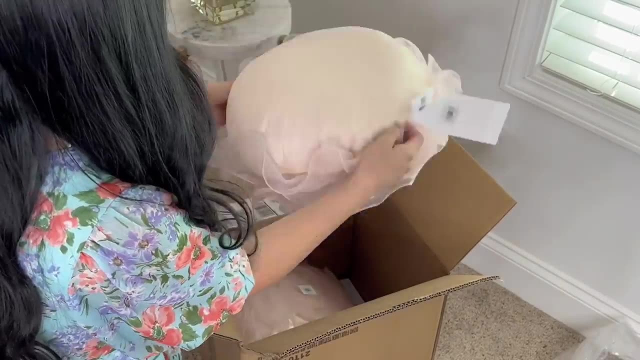 This exclusive back to class promotion I have shared with you all today, where you can save up to 25%. on August, the 16th, I also picked this up: Two of these beautiful light pink floral decorative pillows to match the theme of this room, which is a floral garden. 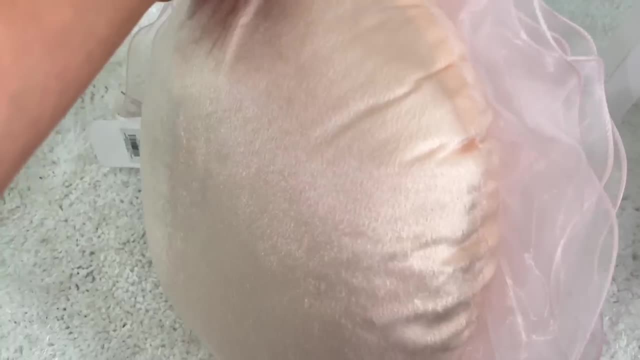 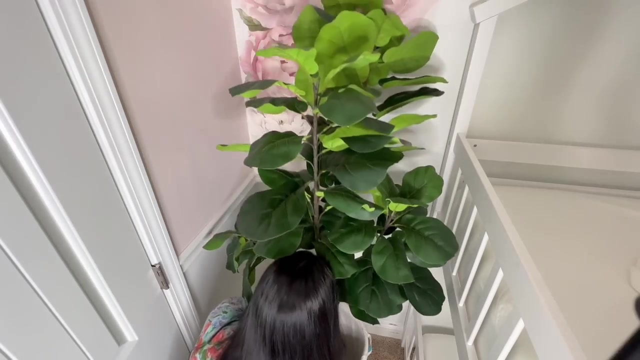 My girls and I love flowers and I love how it ties in with the room together. There has never been a better time to put together a class or room makeover, office space or complete home furnishing update, To check out the items I've shown here today and to browse the vast assortment of on-trend products across different styles only on the Home Depot. 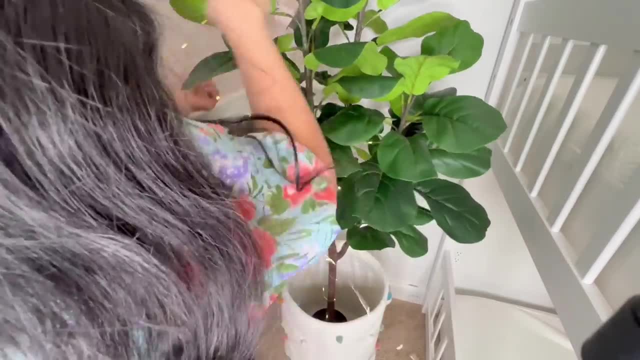 make sure to click the link in my description box. I can assure you will definitely find the perfect pieces to help you complete your next project, as it did for mine. Now let me show you how it all came together. There are two in total here. 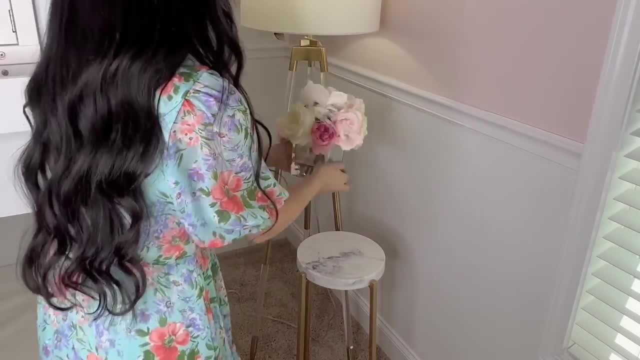 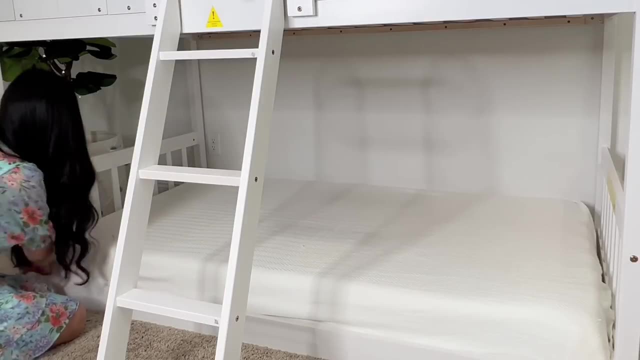 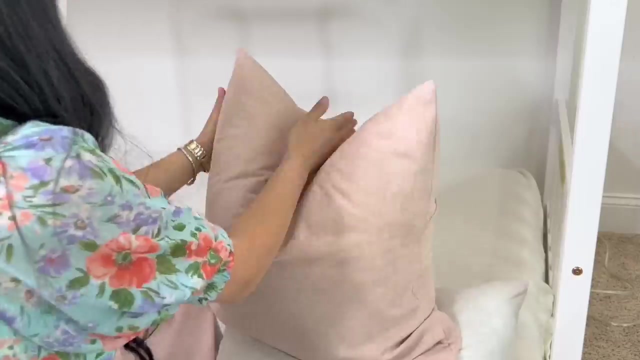 One of the cat-shaped, two of the cat-shaped and one of the boxed and one of the boxed. and If you look at the box here I've got some meeting items. The first one is the first one. I've got my social media account, which I'll put in the video description box for you guys. 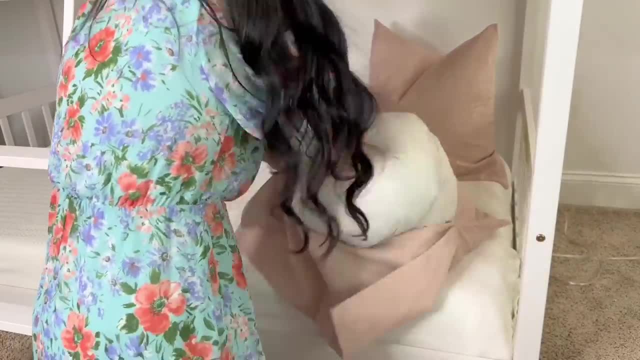 Then it's the other one. This is my Facebook account. I'm on Instagram, Instagramcom and Instagramcom. Here's the link for my social media account. Here's my Facebook account. Three tabs here. I've got my WhatsApp account. 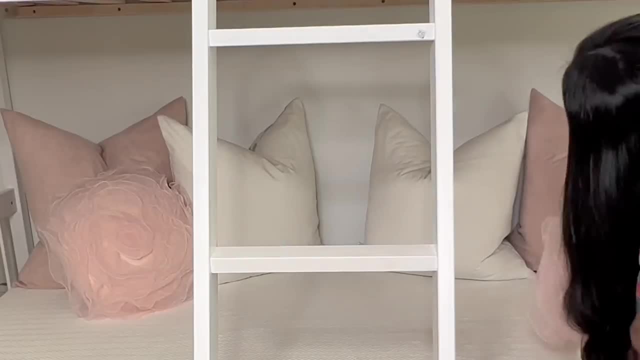 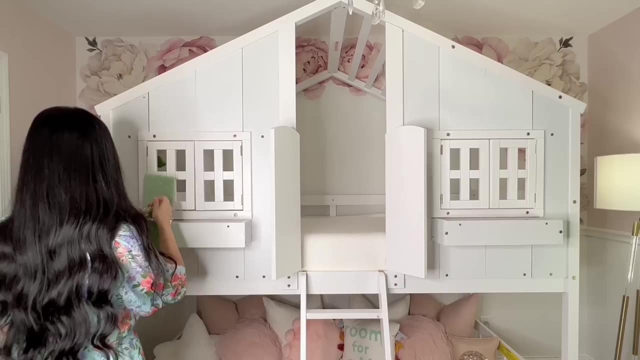 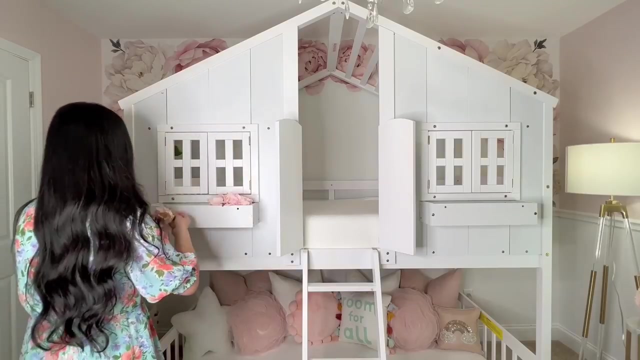 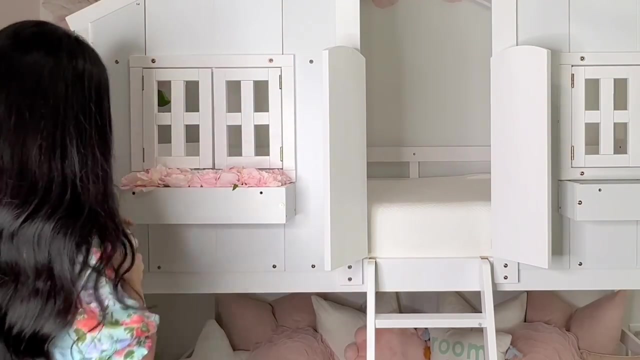 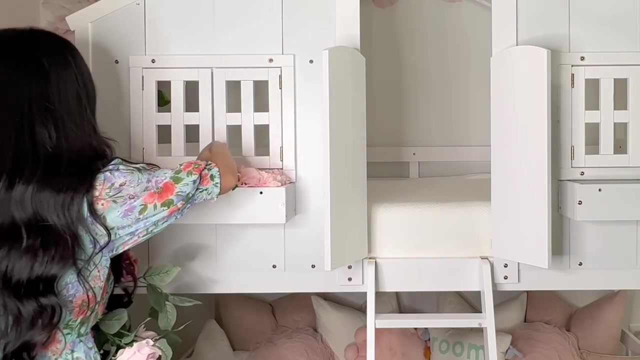 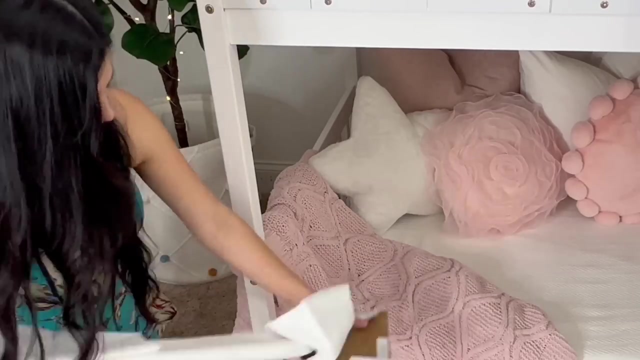 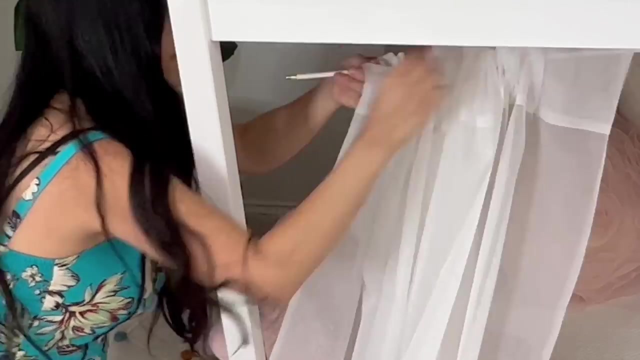 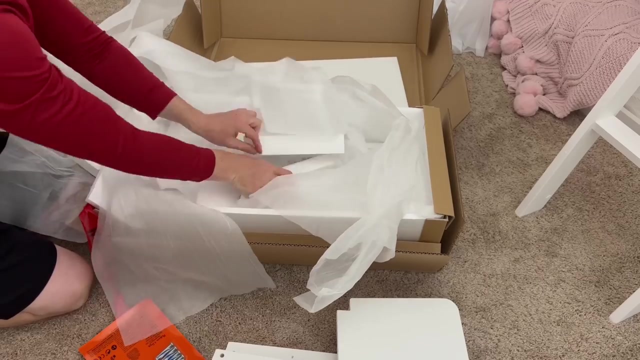 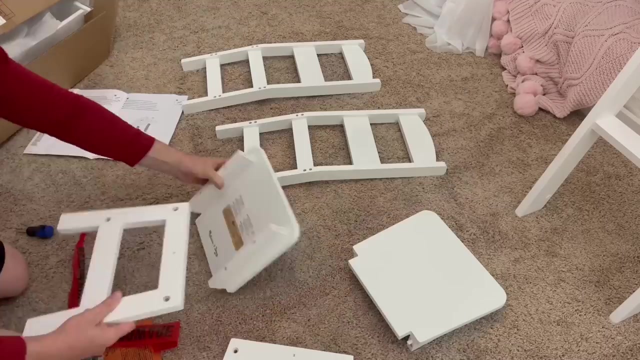 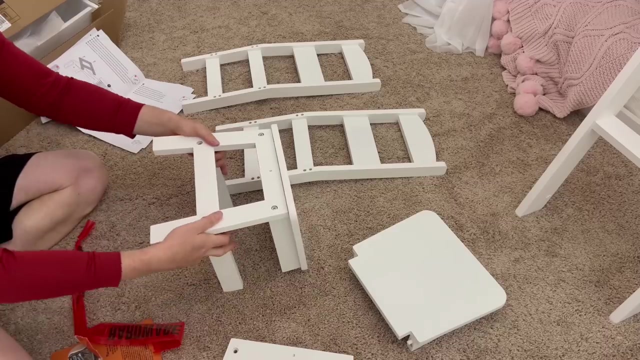 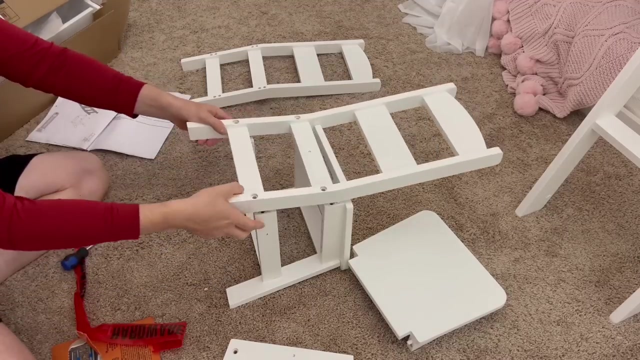 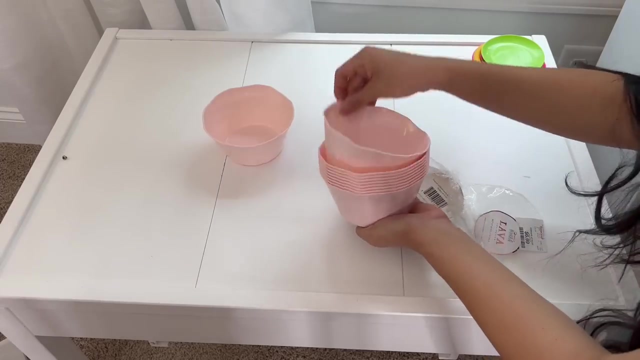 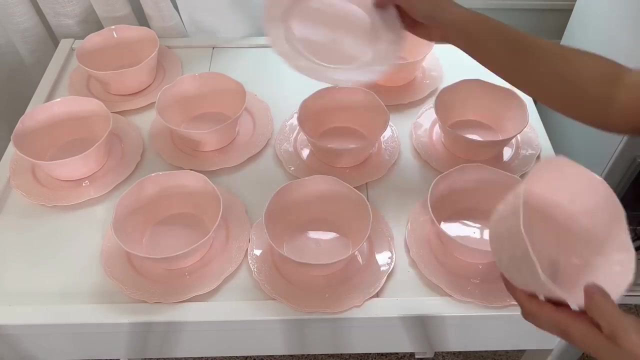 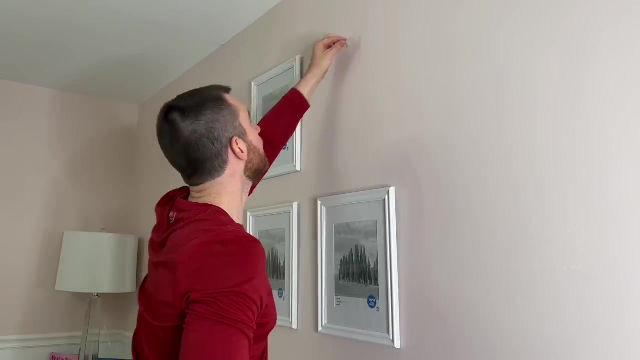 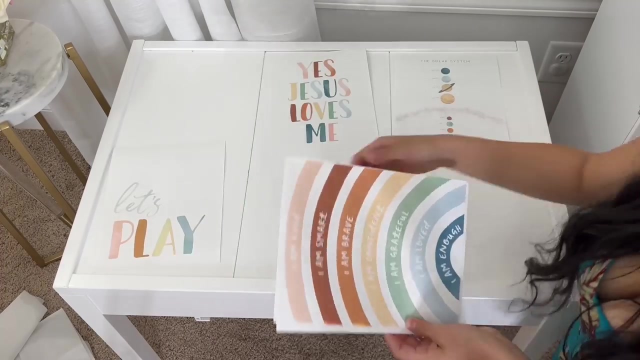 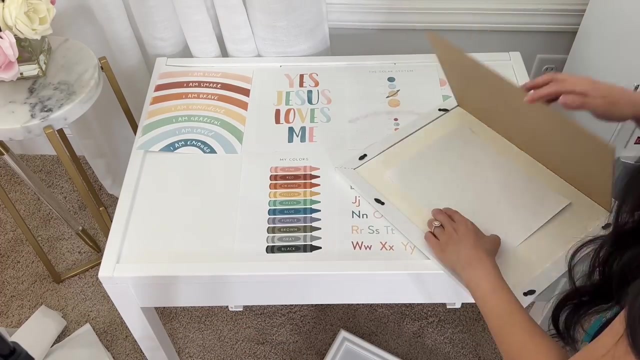 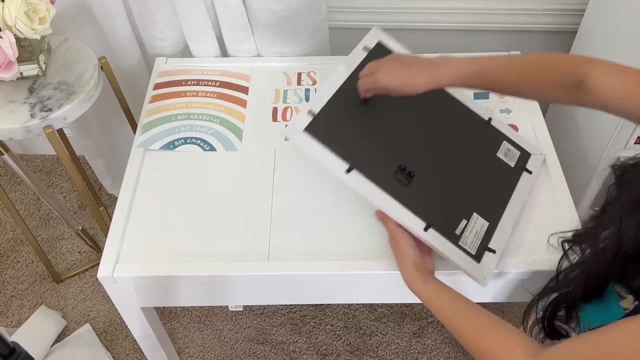 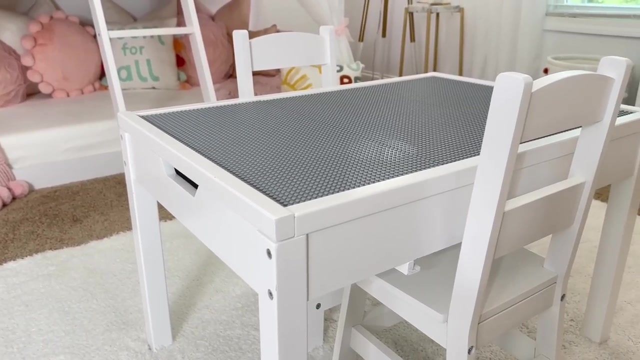 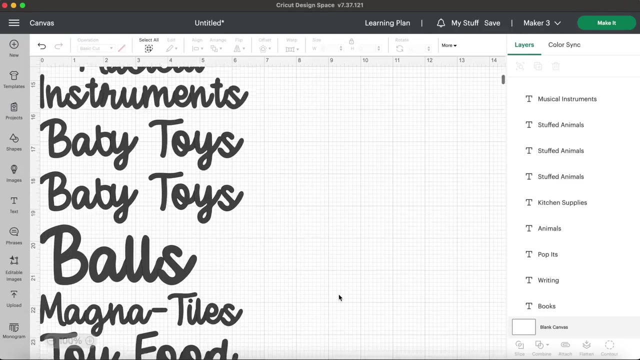 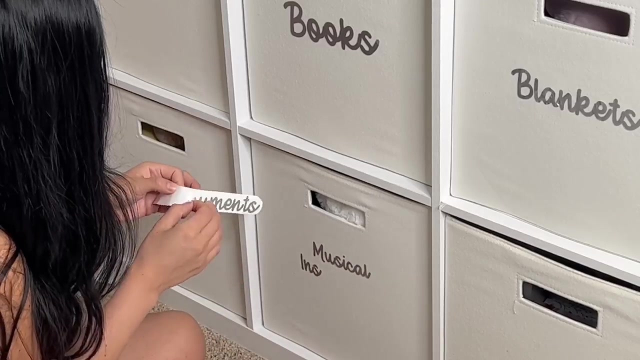 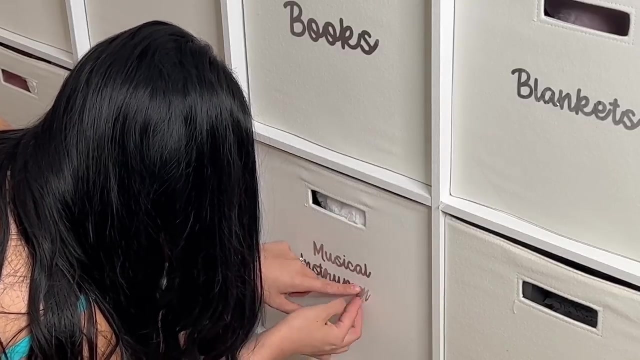 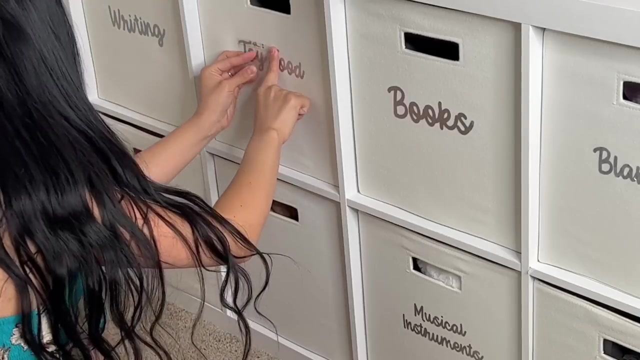 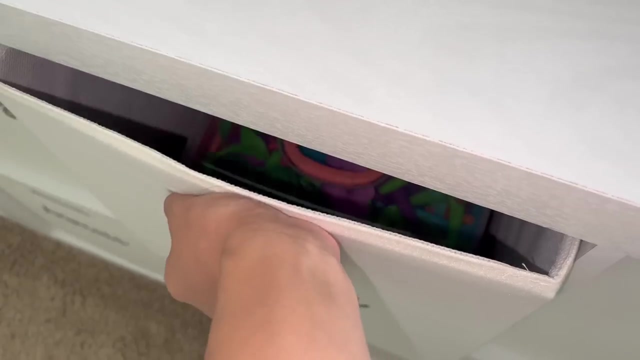 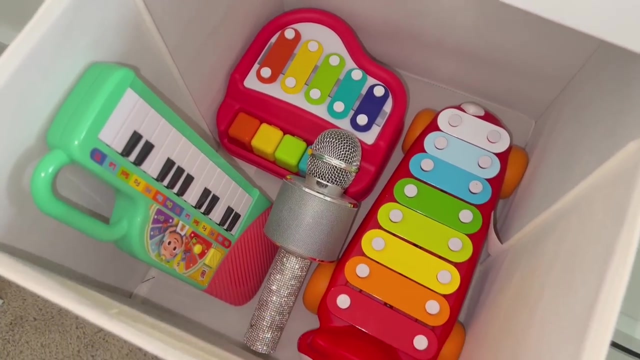 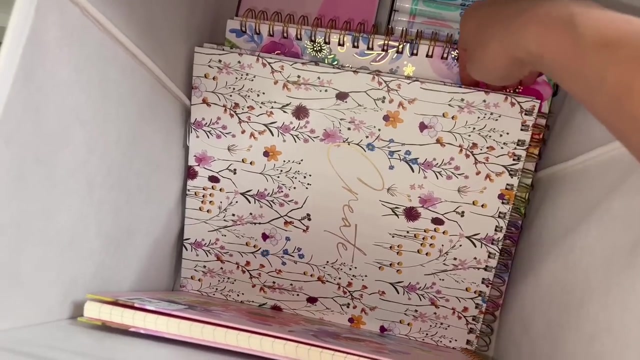 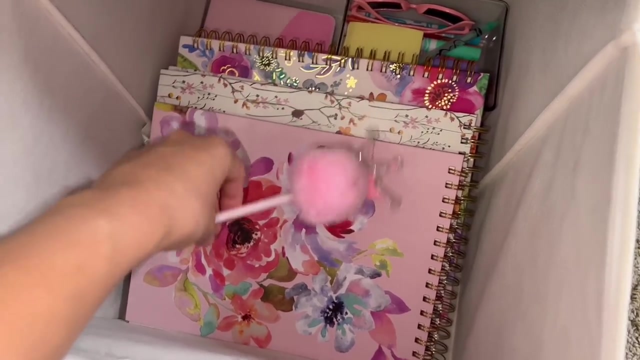 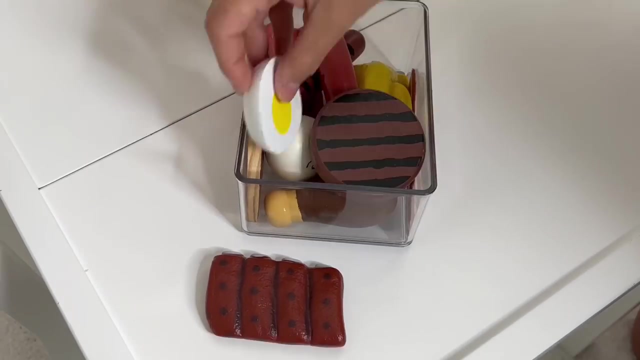 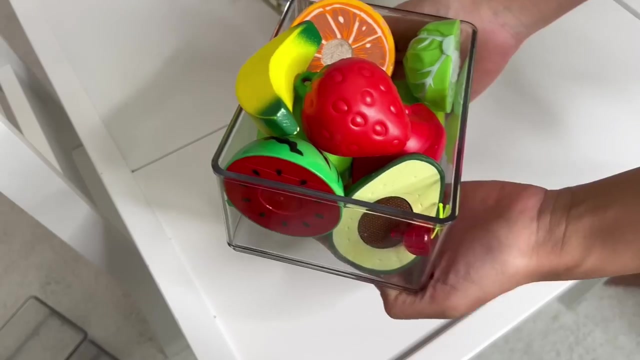 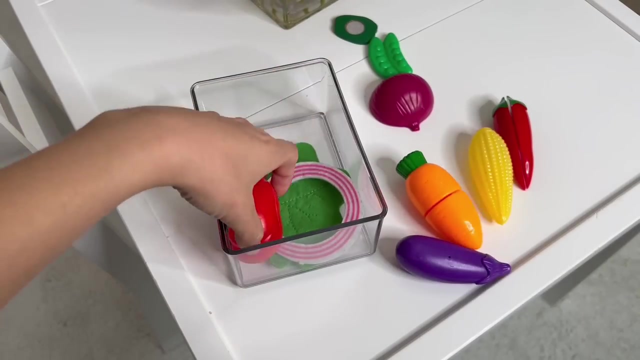 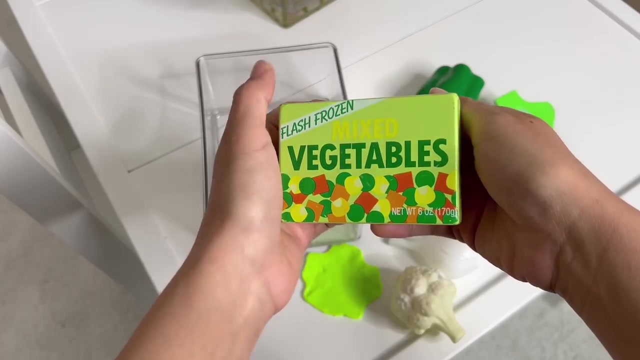 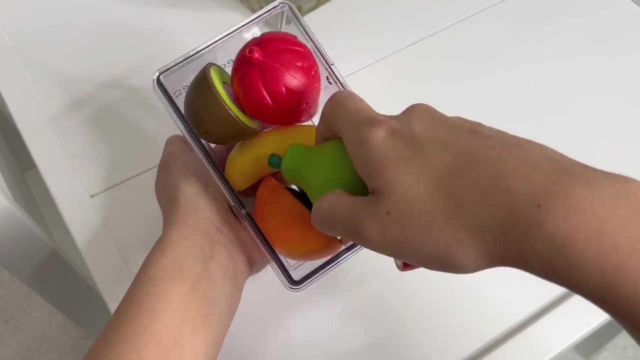 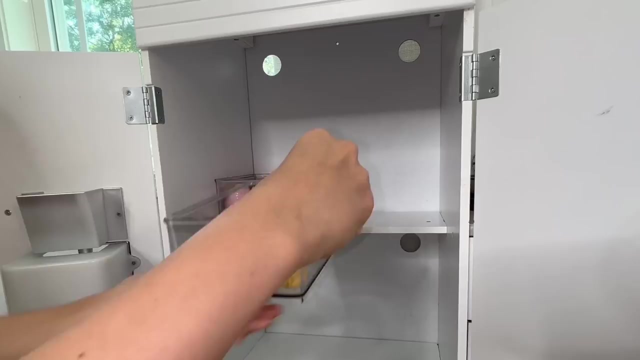 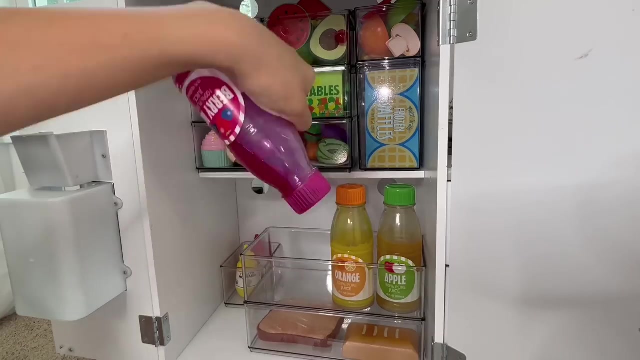 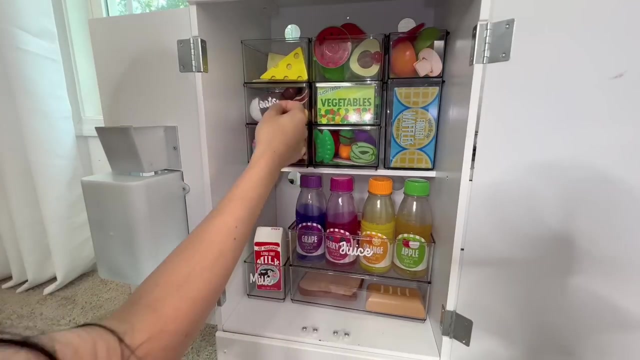 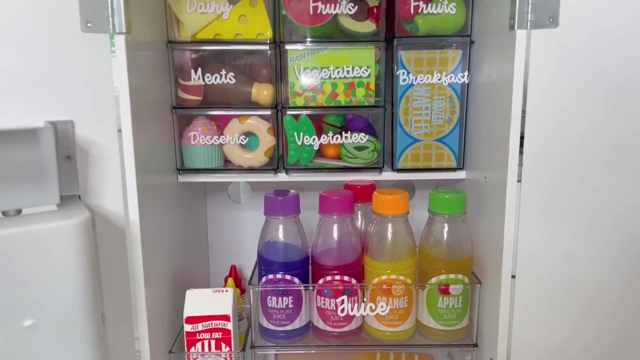 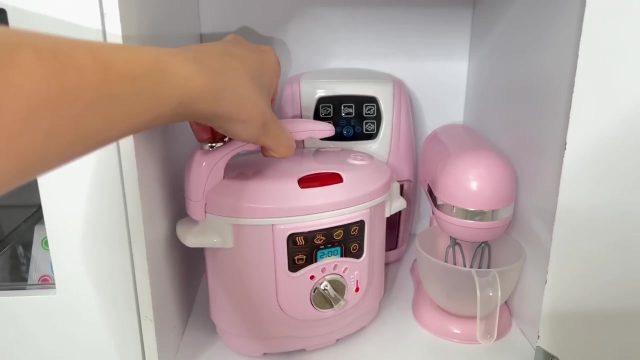 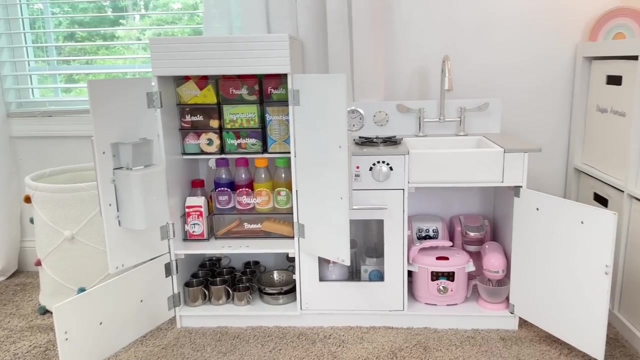 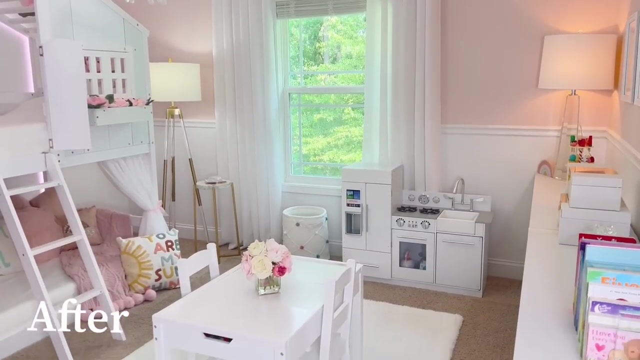 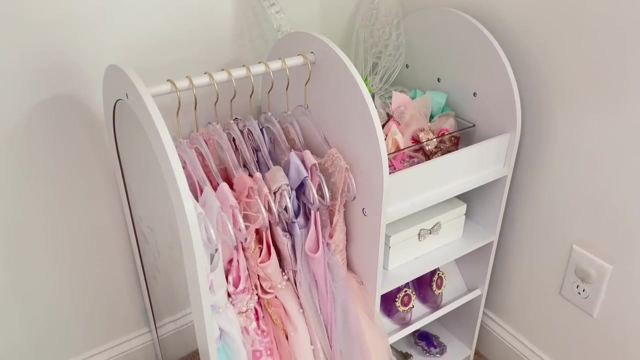 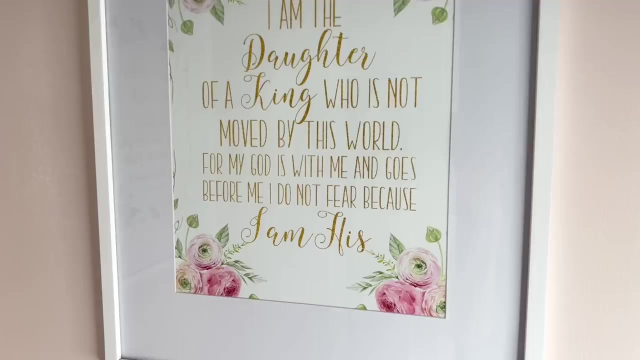 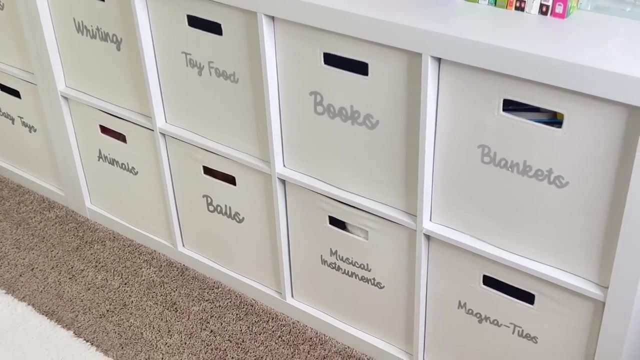 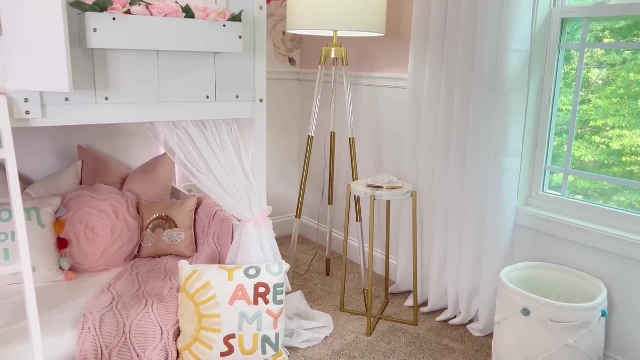 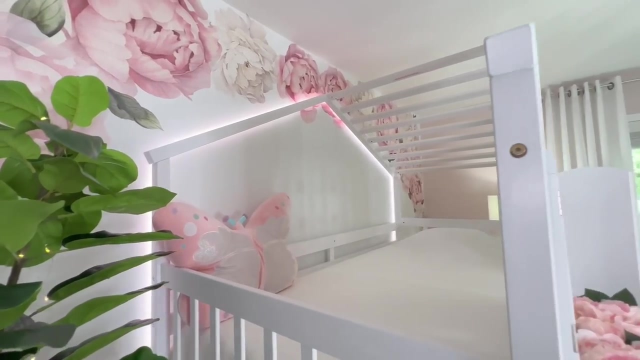 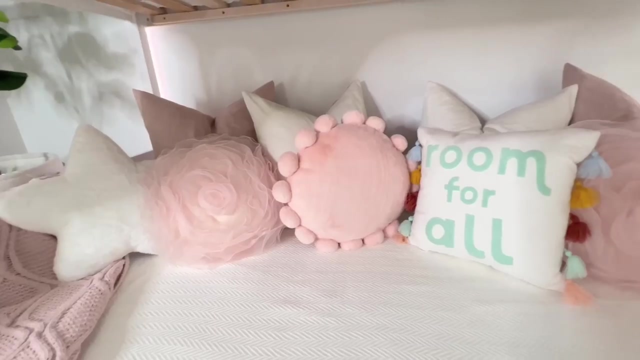 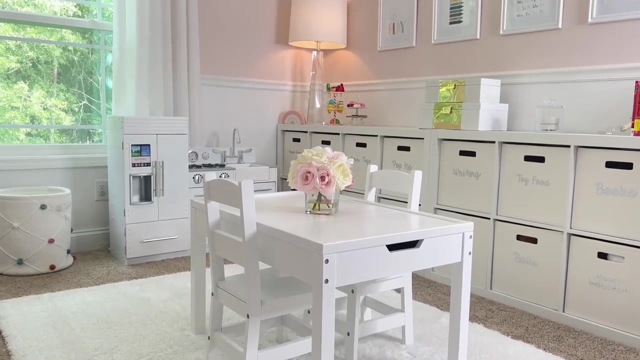